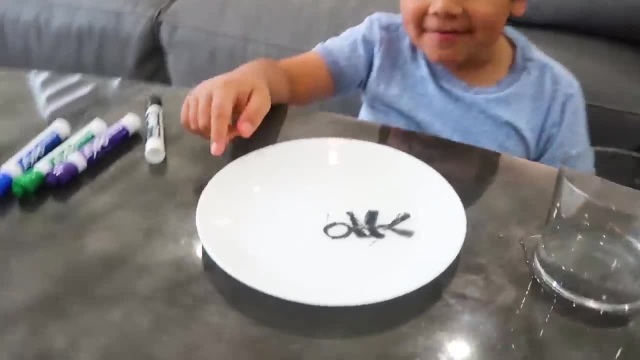 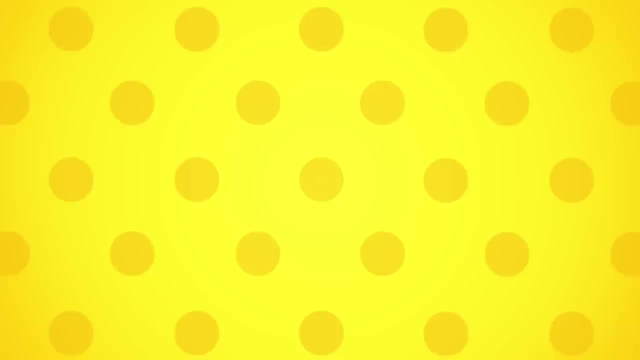 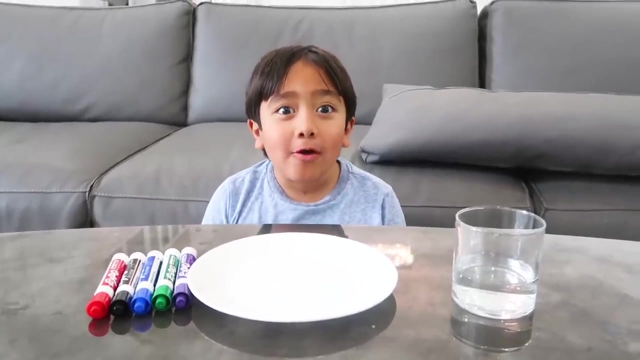 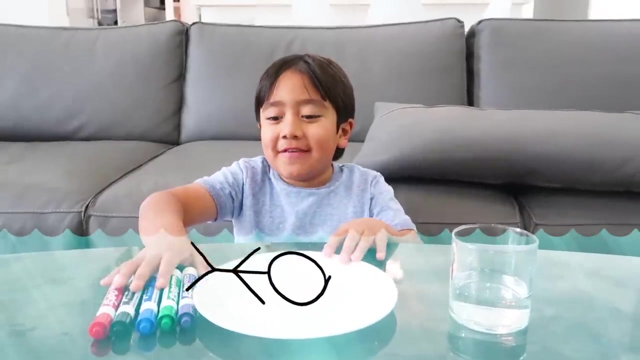 Here we go. This is an easy way to make your stick figure float. He broke. Welcome to Ryan's World. Hi guys, today we're gonna put our trawling and then make it float on water. So this is very easy. All you need are some markers. 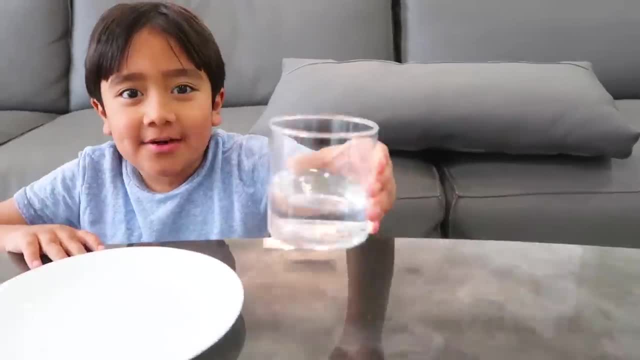 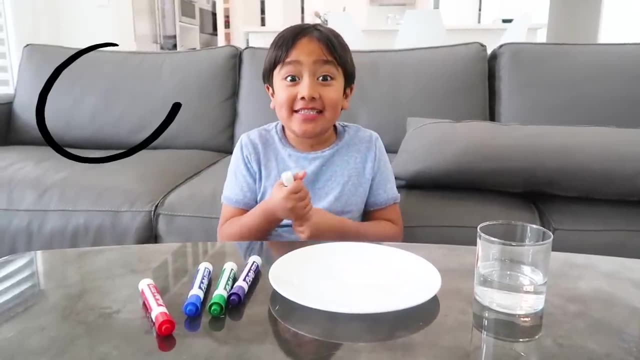 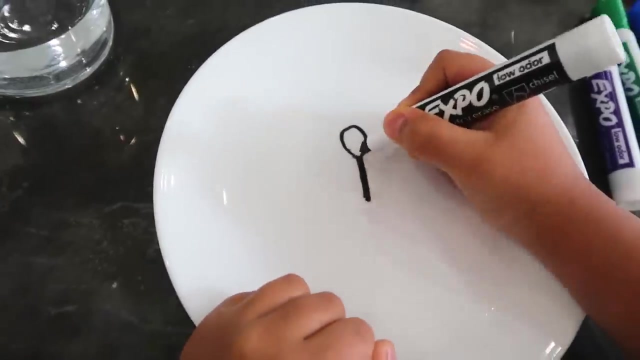 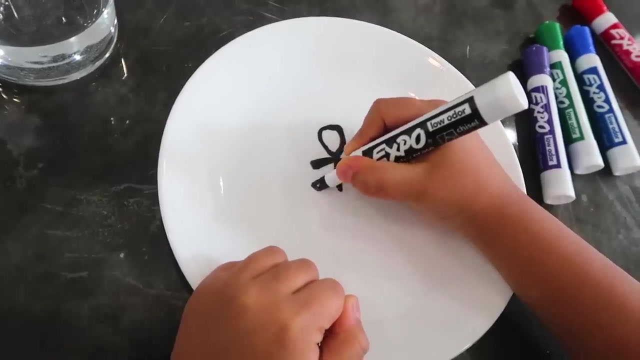 A plate and some warm water. First, draw what you want on the plate. Well, I'm gonna make a stick figure with multiple arms. So like this. Then you make it really thick, Like this, And you make arms And then you make the legs. So after you make your draw, 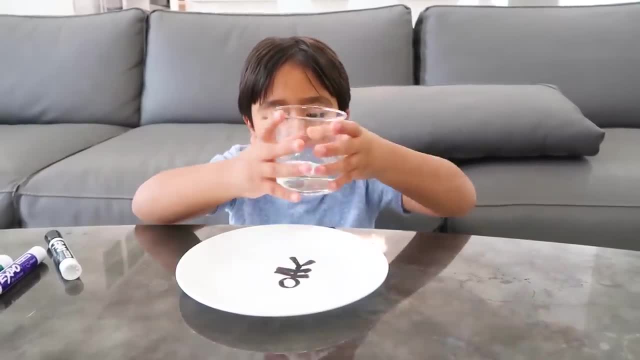 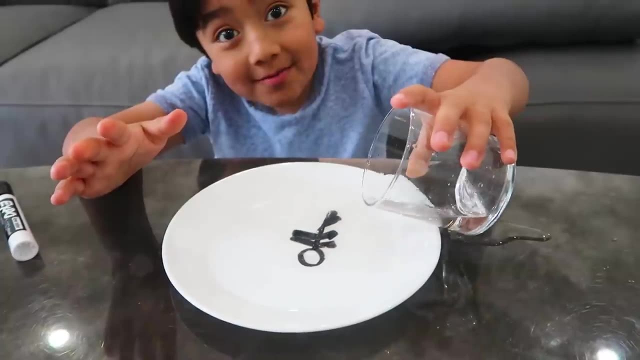 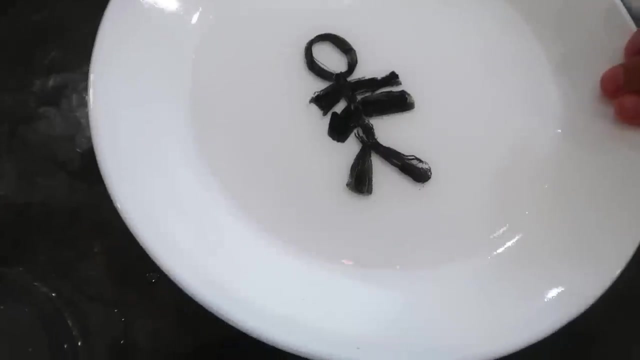 you're gonna start drawing. Then you put some warm water on this side. Whoa, He moved. Look he's dancing. Oh, his arms too. I feel like the arms or legs are gonna break. Oh, it's moving now. Yay, Now he can just walk. 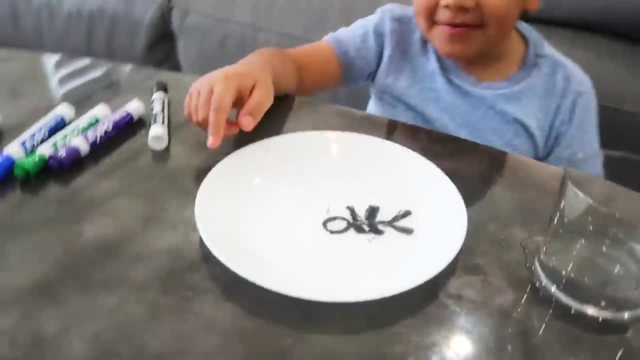 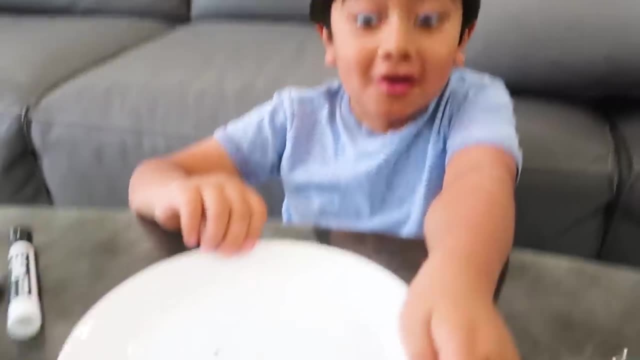 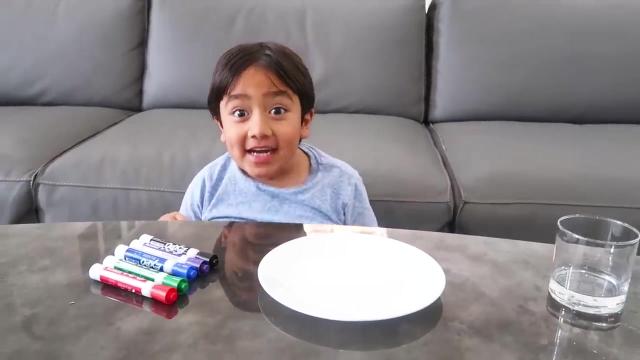 There you go. This is an easy way to make your stick figure float. Oh, He broke. This is so cool, You can hold it. Okay, guys, for the next one, I'm gonna make a dog. It should be like this. 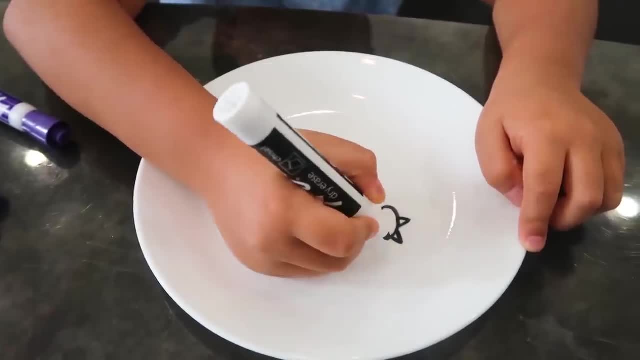 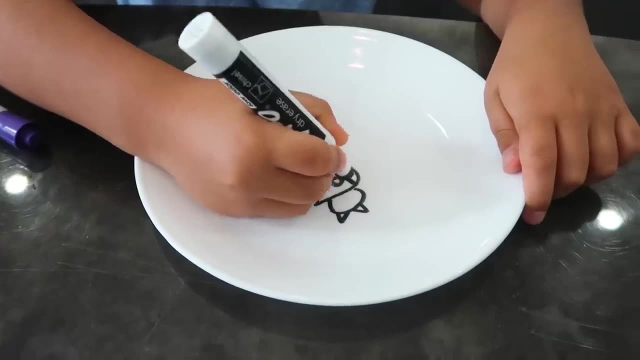 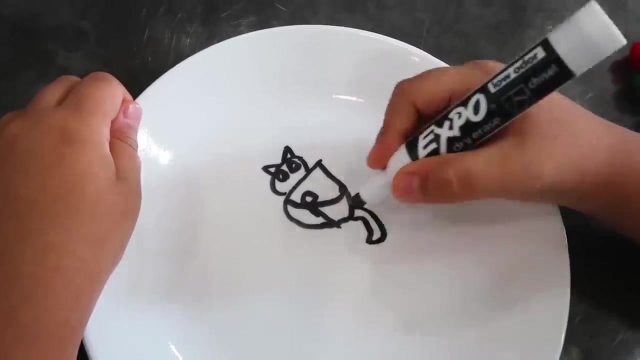 And then maybe I can put like ears. I feel like I'm making a cat. I'm making a big dog or cat. Oh, I can't do it right, Unless I do, like this: I put an R. Okay, then I'll make the legs. 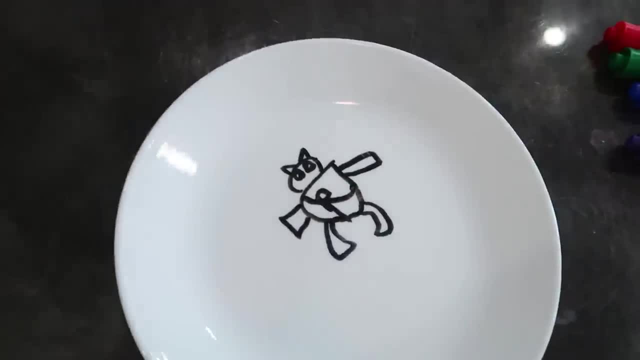 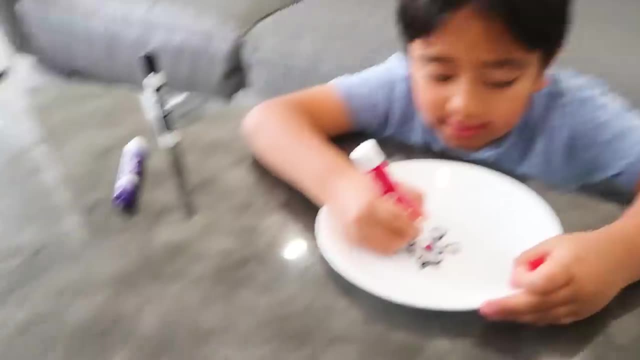 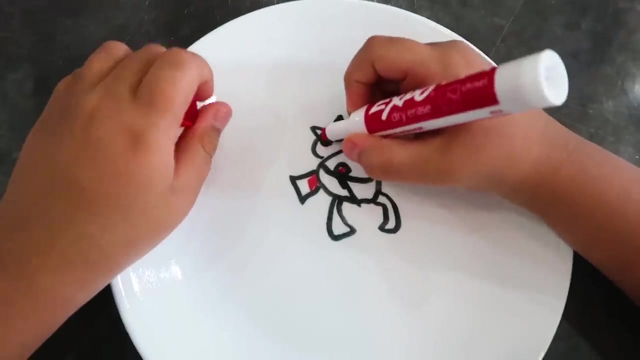 And then the arms. I feel like I'm making like a super strong cat or something Meow. Okay, now I'm going to put red right here And then I'm gonna make this red And then I'll make the eyes red.